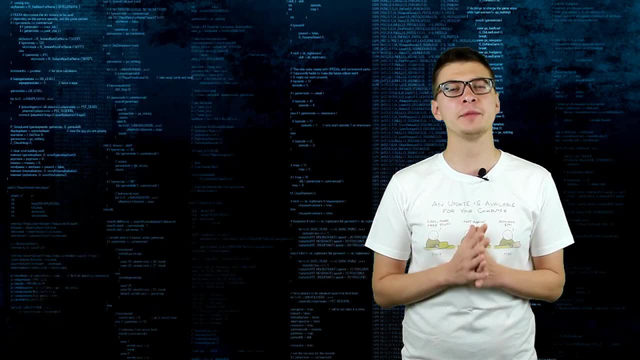 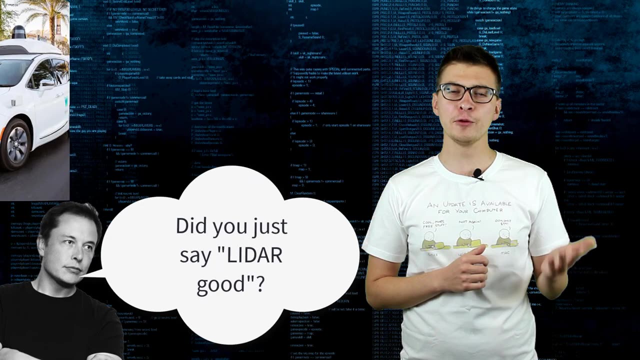 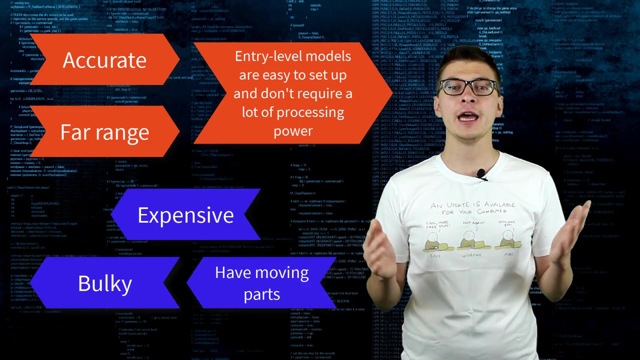 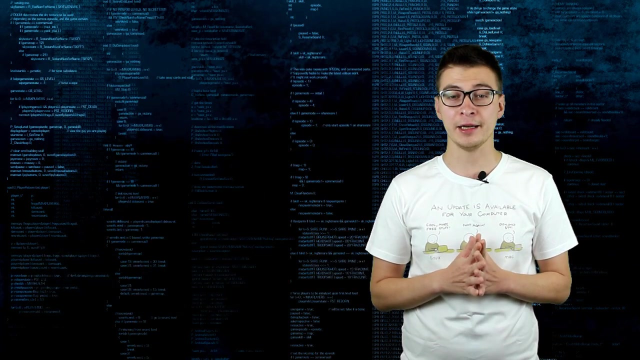 slam is relatively easy to set up and it is quite precise. there is a reason way my uses lighters on their self-driving car, but of course there is a reason that Tesla doesn't. lighters are bulky, quite expensive and since they have rotating parts which require maintenance when in operation for long periods of time for 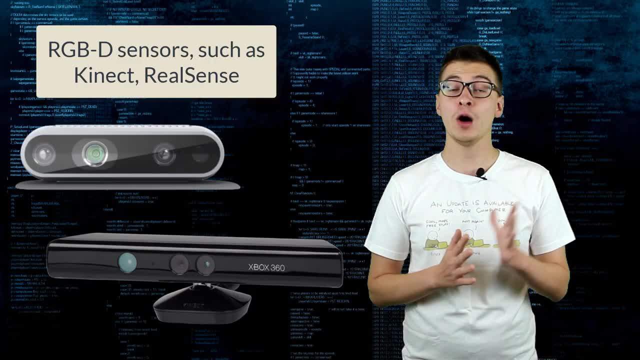 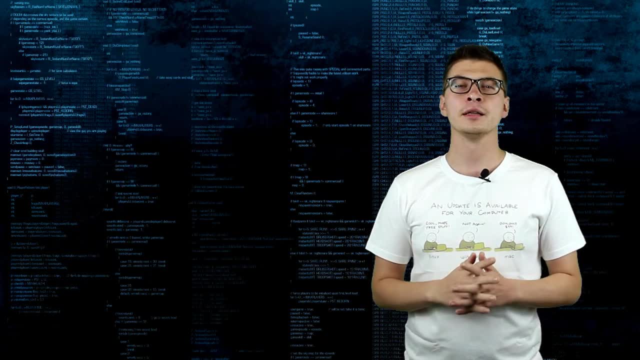 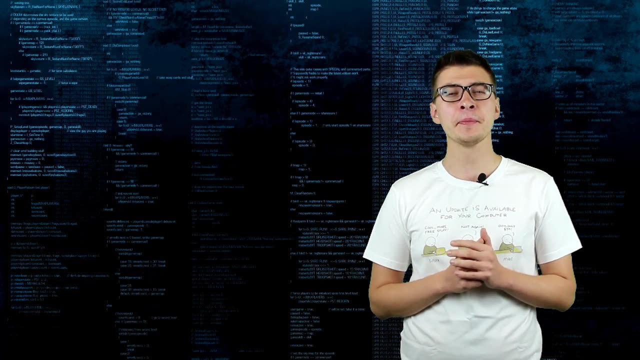 visual slam. our GPD sensor approaches also can be quite robust. we are a simple stereo or monocular systems are tricky to set up. you new but more borders will see then. I Manoj some links in the video description so you can read about slam in more detail. 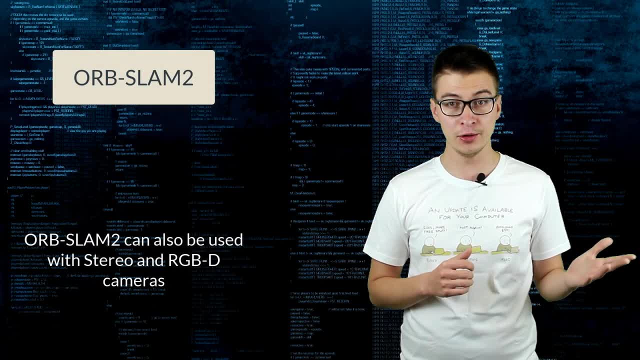 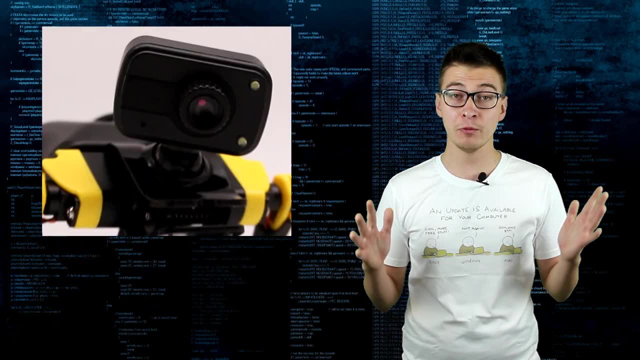 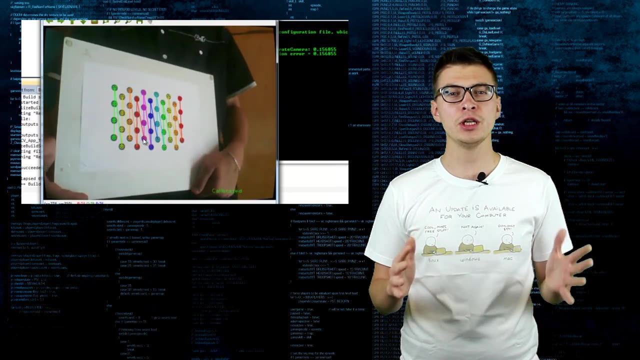 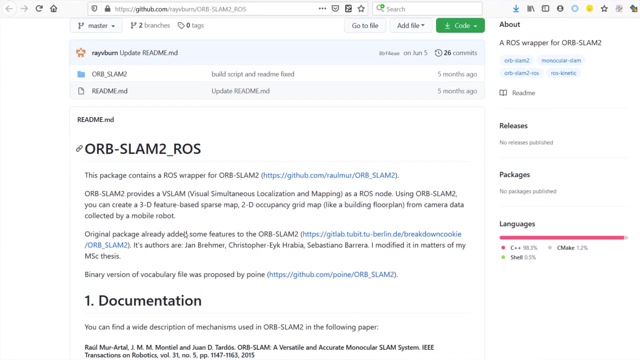 for today's video. we'll use monocular visual slam algorithm called orb slam to you and a lighter based Hector slam for orb slam to. we will use regular chip web camera. it needs to be calibrated to determine the intrinsic parameters that. read more about camera calibration in the accompanying article. there is a. 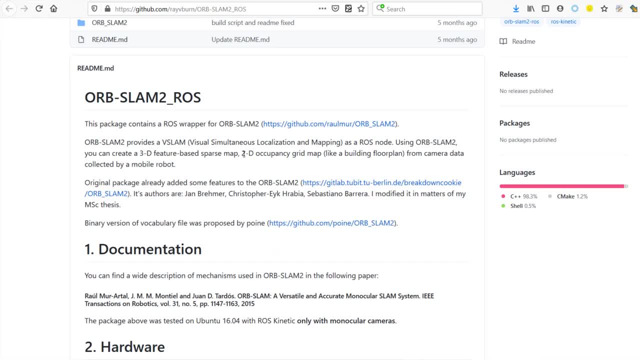 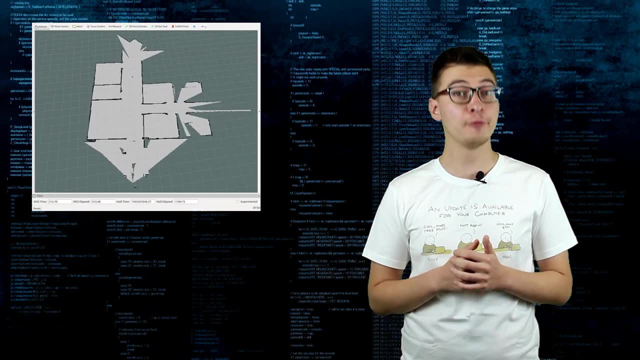 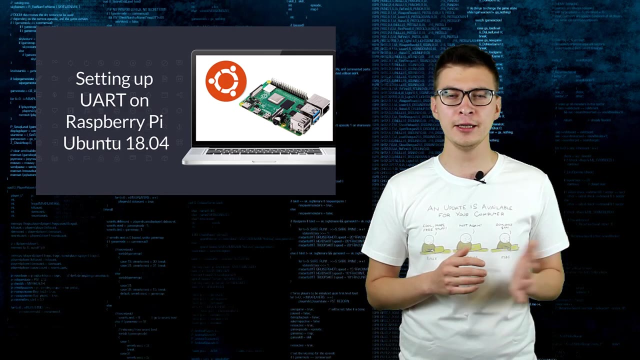 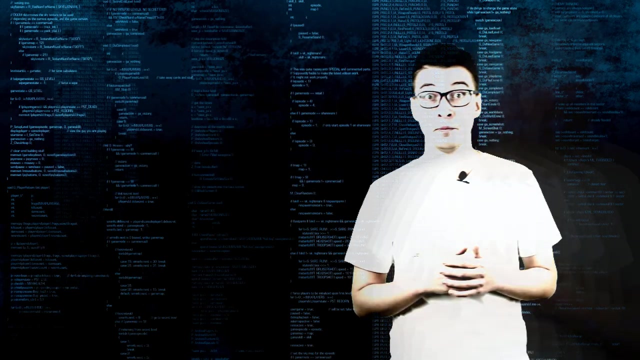 package integrating orb slam 2 with Ross, which also publishes 2d occupancy map which looks a similar to building floor plan. the installation process is quite complicated. I recommend to use Ubuntu 18.04 image for Raspberry Pi as the starting point to avoid the need for compiling many, many, many many additional. 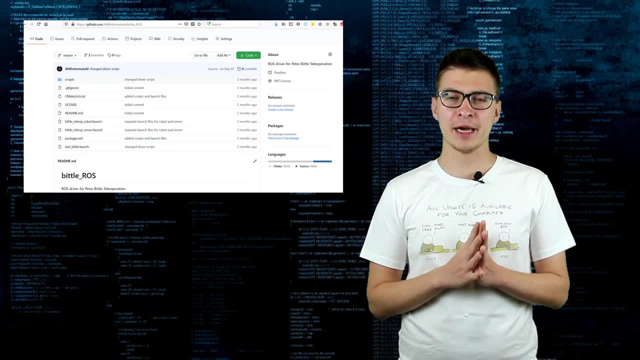 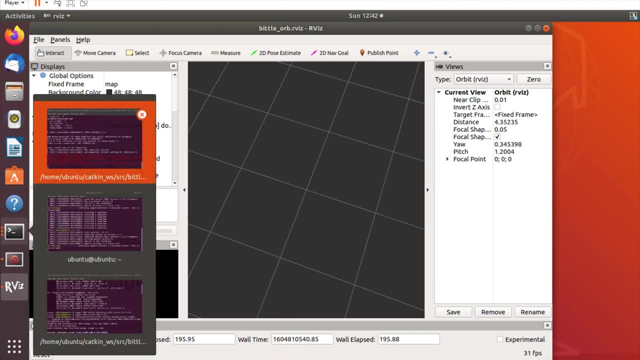 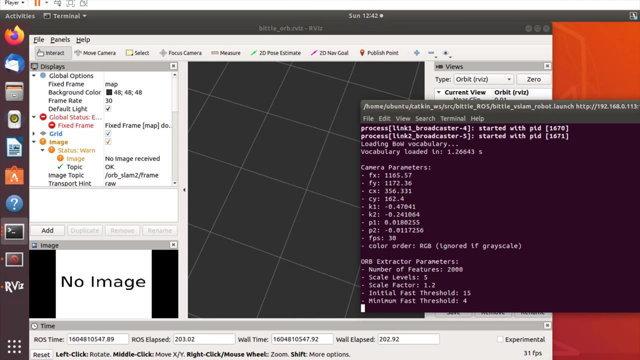 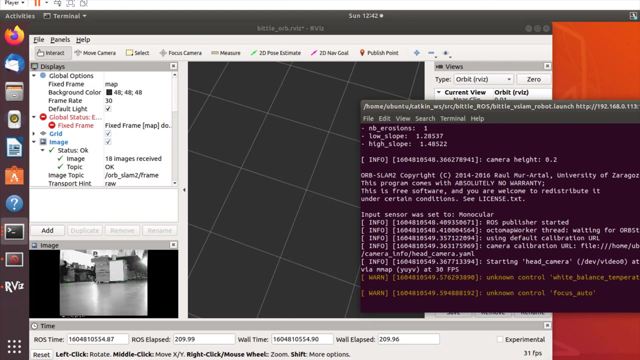 packages. once you have it and packages for beetle you or your robot base web camera drivers installed, you can run beetle underscore, robot underscore V slam dot launch file from my beetle driver repository on github. it will bring up the whole system robot driver web camera node and orb slam 2 node. orb slam 2 requires enough information about. 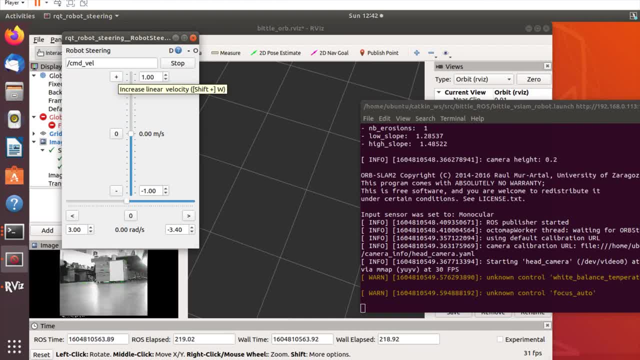 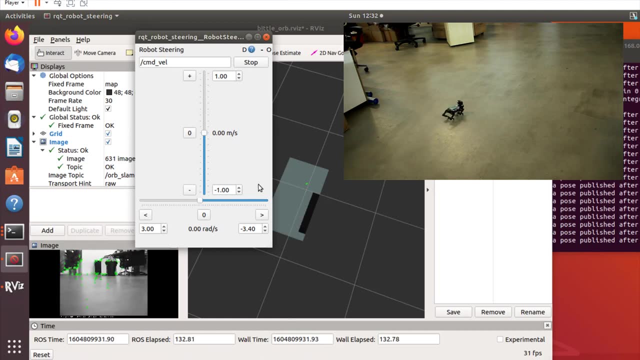 the environments to initialize so you can manually move the robot around to avoid large changes in translation or orientation. after orb slam 2 is initialized, it will start publishing OctoMap or occupancy map. you can use controls now to move your robot around. unfortunately, I found that because the camera on beetle moves too fast during turning it. 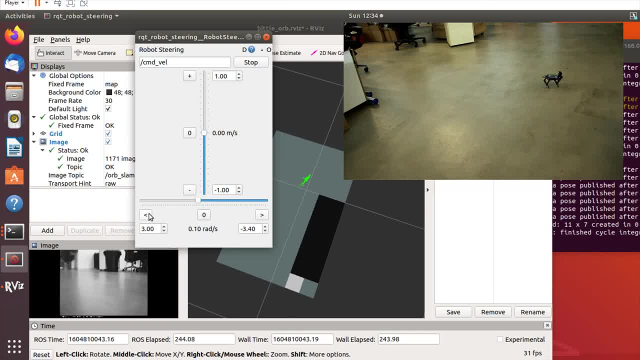 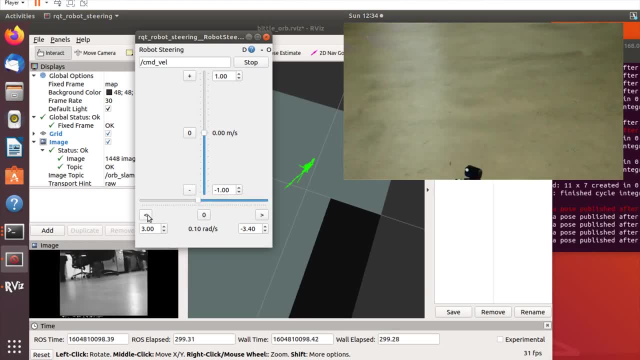 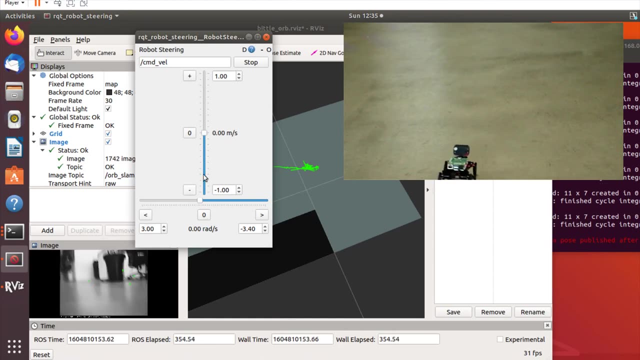 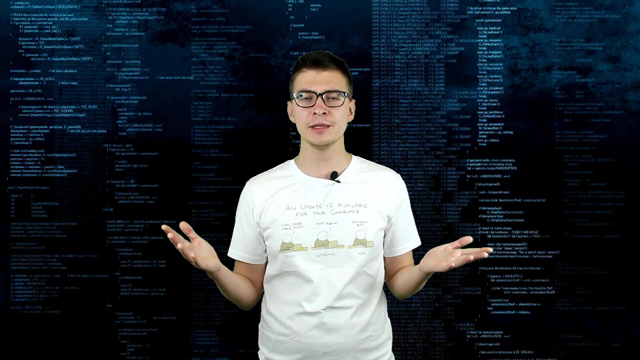 tends to lose the key points and needs to return to its previous position. a couple of improvements that can be made to make it more stable is using a stereo camera. with orb slam 3, it is possible to integrate IMU data for more precise positioning, if visual slam didn't really work for our robot. 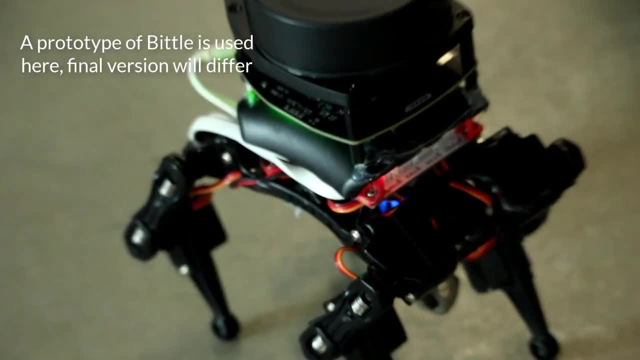 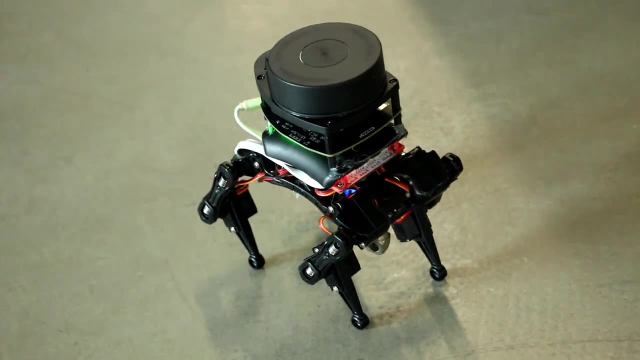 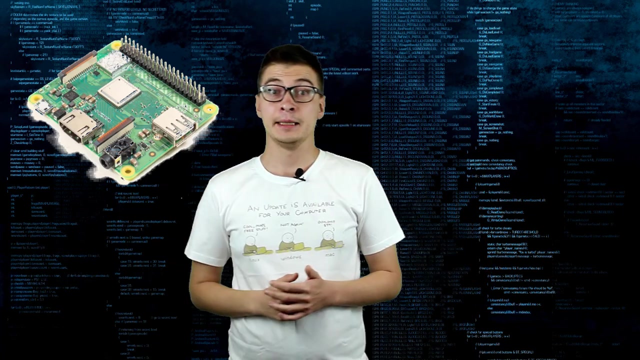 how about installing lighter and trying out one of the laser scanner based algorithms? good news here is that for lighter we wouldn't need as much processing speed, so we can use older Raspberry Pi 3 model which fits nicely on beetle. the bad news is that even a small either is big- the one I had at my 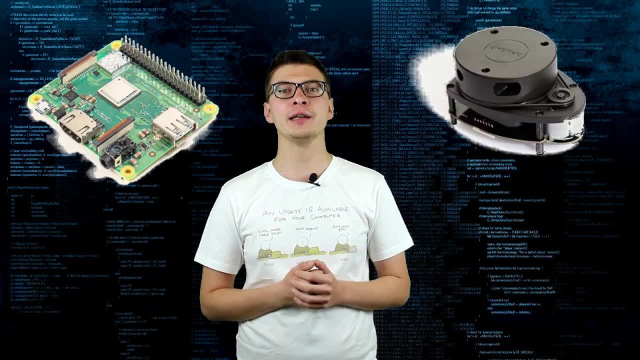 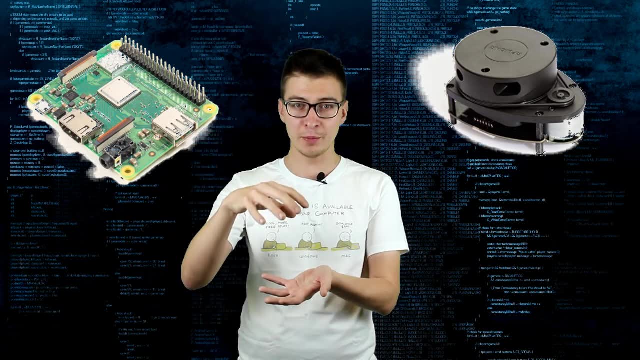 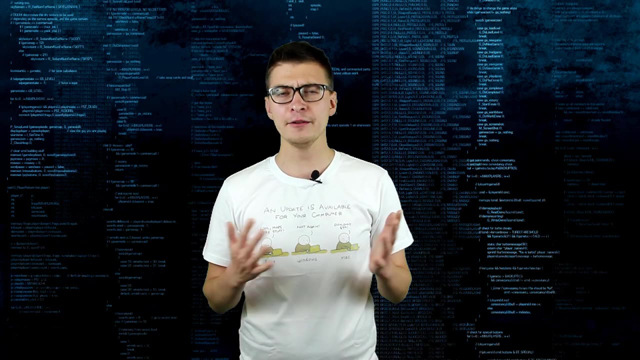 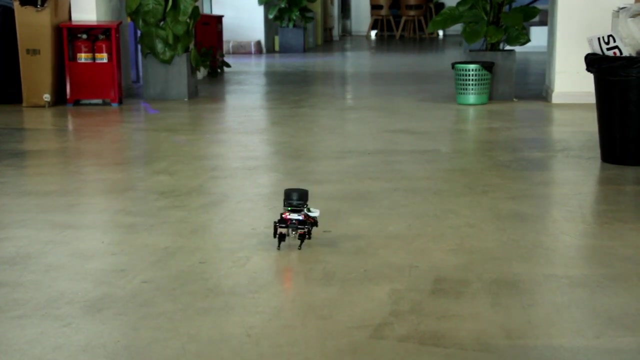 disposal was RP lighter a1m8. it weighs about one hundred ninety grams which, when mounted on top of this leg robot, seriously disturbs its gravity center and influences the walking gait. after adding some additional weights to balance things out, it could crawl and walk, albeit I was still trying to be careful and avoid sudden stops. software. 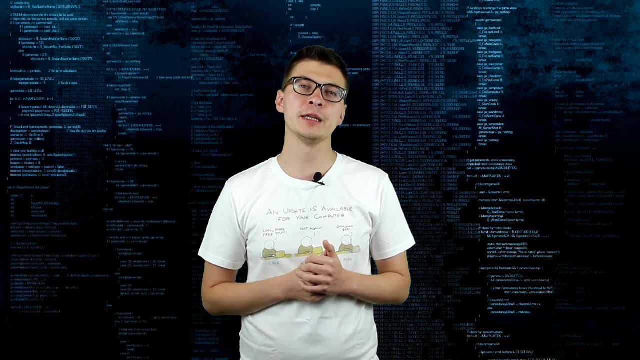 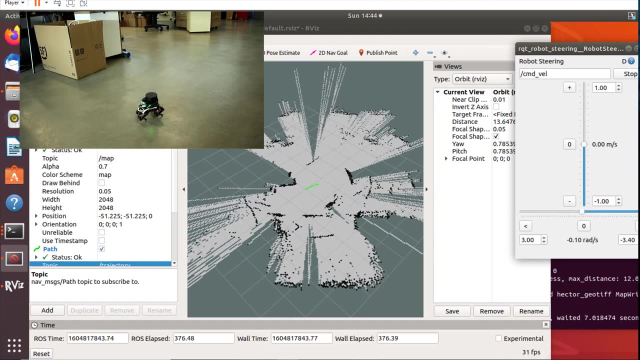 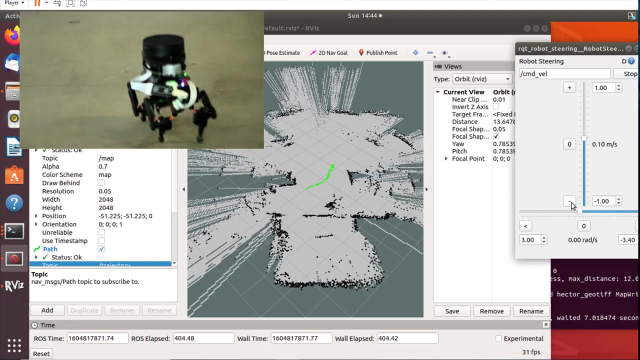 installation for Hector slam is a breeze on Ubuntu 18.04. after it's installed, run beetle underscore, robot underscore, L slam dot launch file to bring up lighter robot control and Hector slam node. overall mapping results look much better than with orb slam 2, and Hector slam can even publish odometry and pass messages.